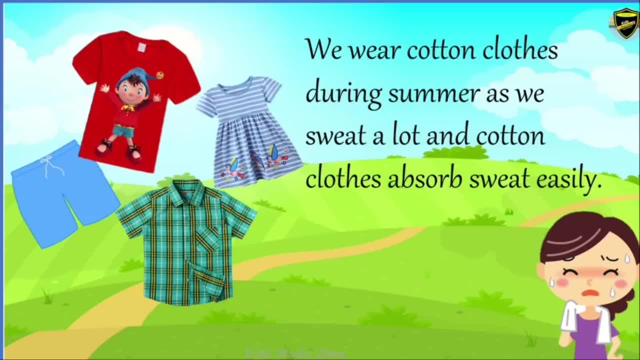 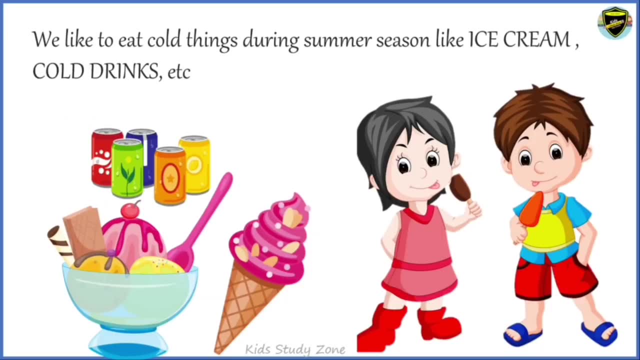 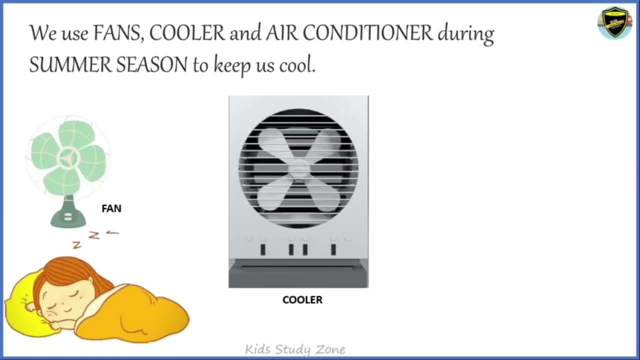 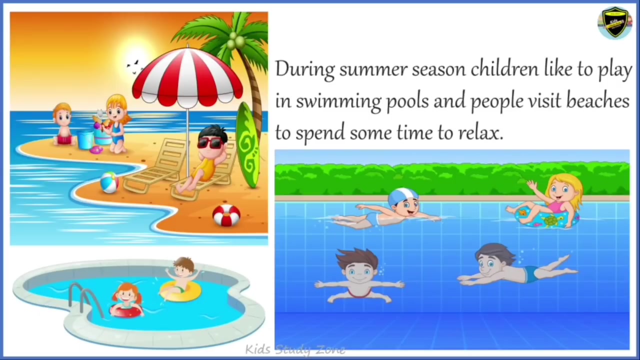 frock and lower. We like to eat cold things during summer season, like ice cream, cold drink, etc. We use fans cooler and air conditioner during summer season to keep us cool. During summer season, children like to play in swimming pools and people visit beaches to spend some time to relax. 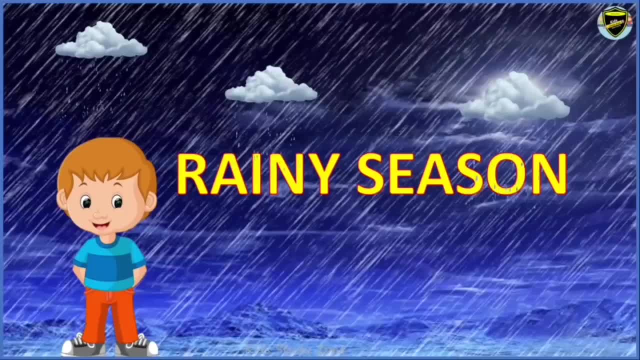 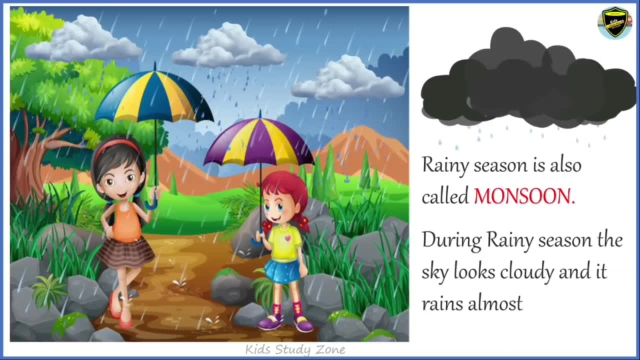 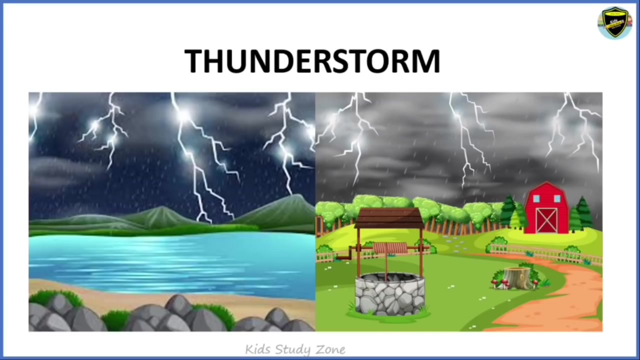 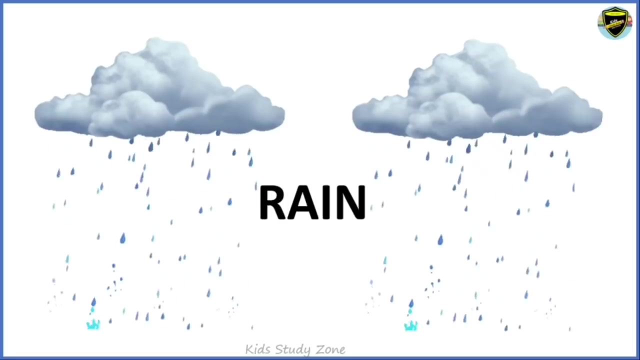 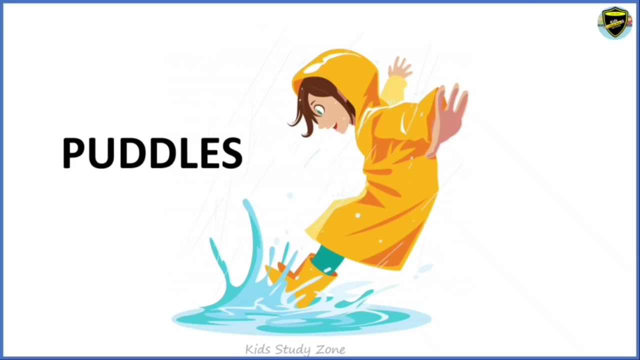 Rainy season. Rainy season is also called monsoon. During rainy season, the sky looks cloudy And it rains almost every day. Things we see during rainy season: Thunderstorm, Dark clouds, Rain, Rainbow Puddles. Now let's see the things. 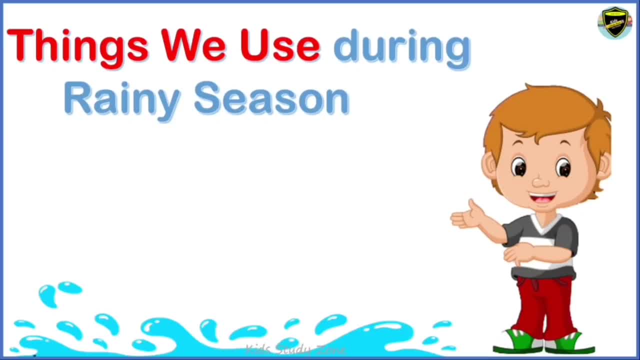 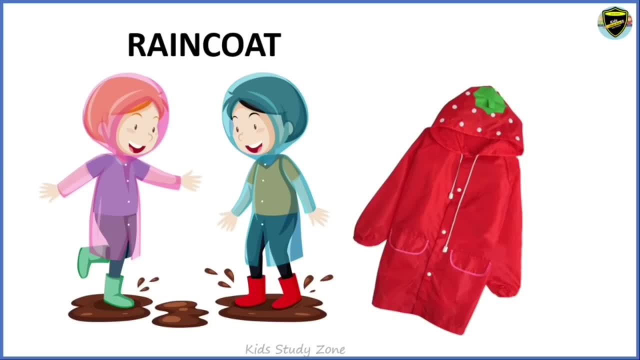 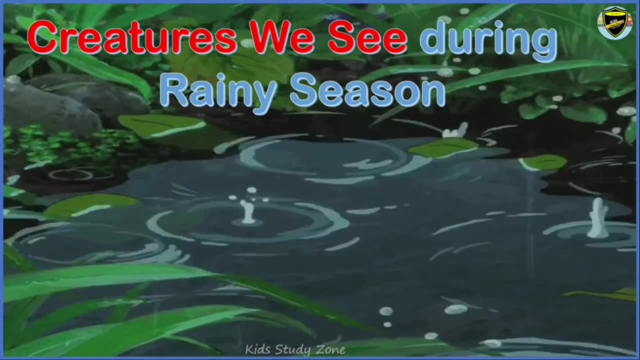 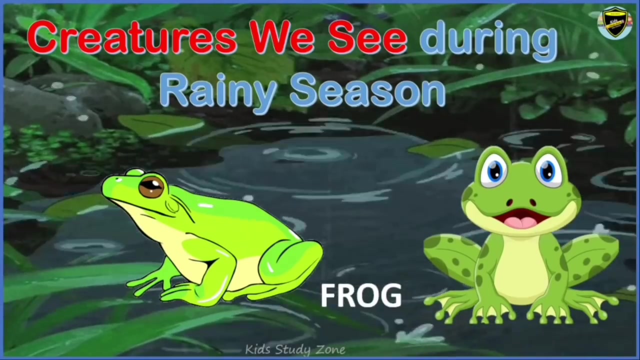 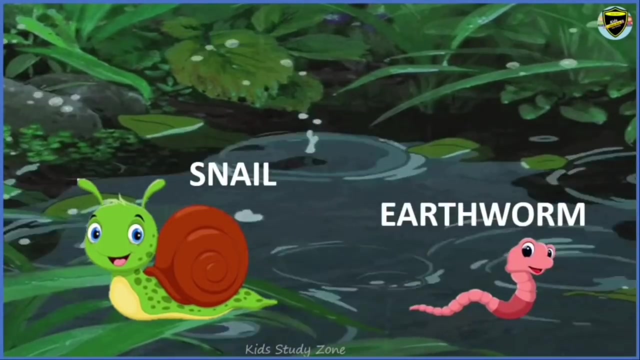 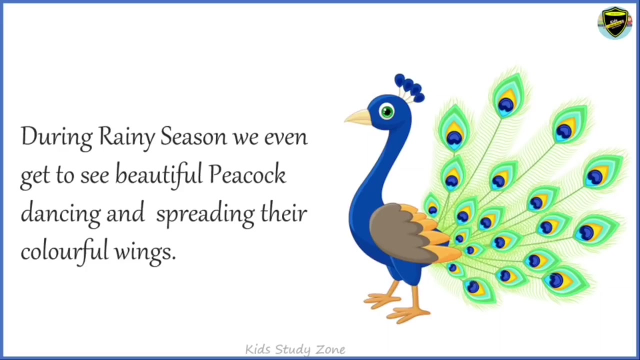 Things we use during rainy season: Umbrellas, Gum boots, Raincoat. Now let's see the creatures we see during the rainy season: Frog, Snakes, Snakes, Snakes, Whale, Earthworm. During rainy season, we even get to see beautiful peacock dancing and spreading their colorful wings. 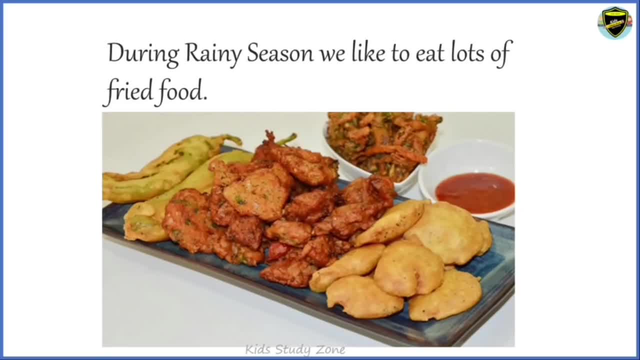 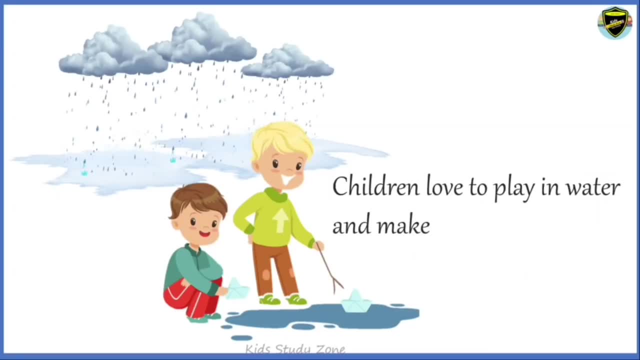 During rainy season we like to eat lots of fried food. Children love to play in water and make paper boards. Children love to play in water and make paper boards. Children love to play in water and make paper boards- Winter season. It is very cold and chilly during winter season. 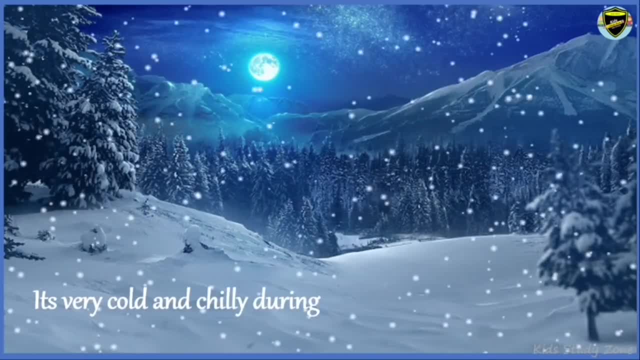 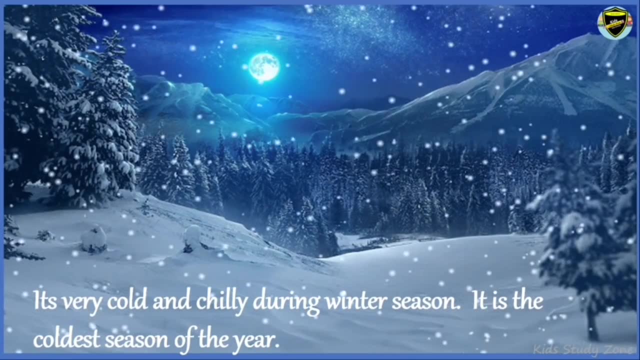 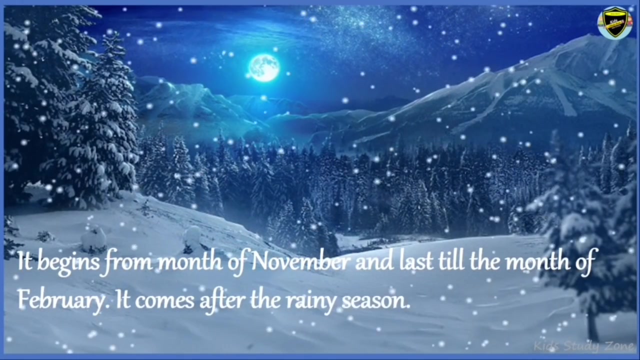 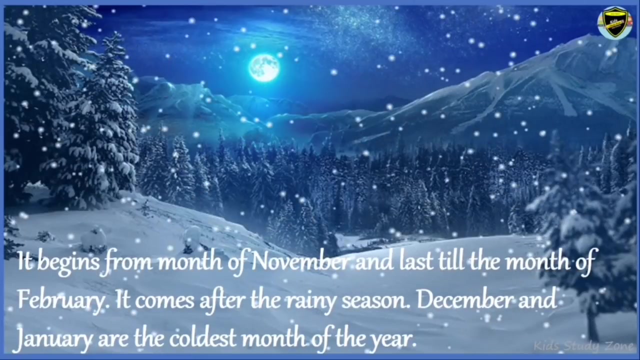 It is the coldest during the winter season. It begins from the month of November and lasts till the month of February. It comes after the rainy season. December and January are the coldest months of the year. The days are shorter and increases by two. 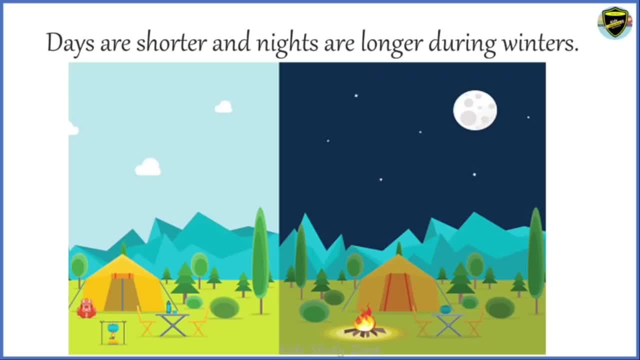 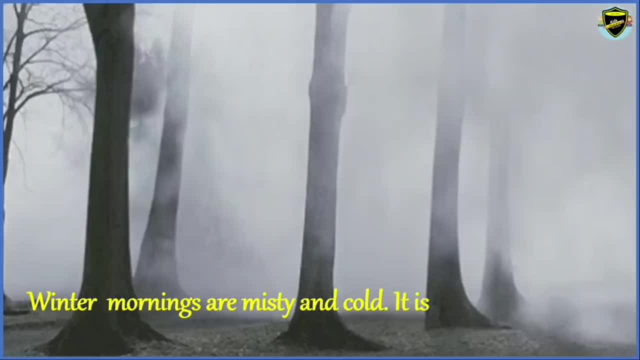 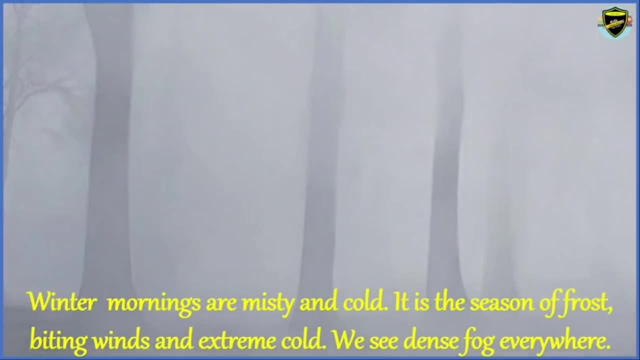 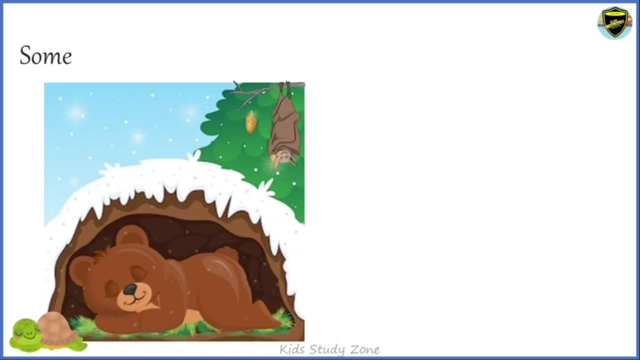 So that you just must enjoy. the place are shorter and nights are longer during winters. Winter mornings are misty and cold. It is a season of frost, biting winds and extreme cold. We see dense fog everywhere. Some animals, like bears, bats, turtles, hibernate during winter. Hibernation is a way animals conserve. 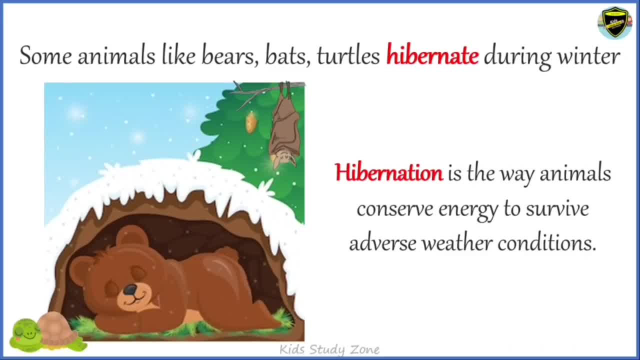 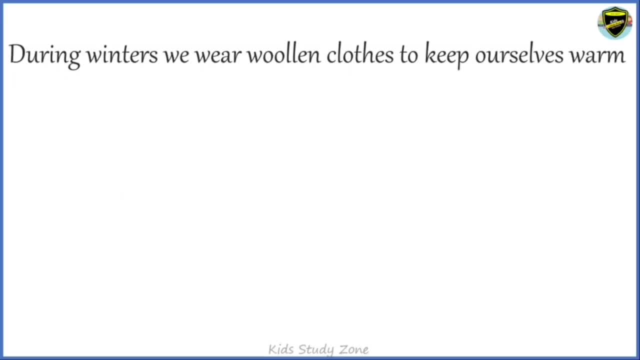 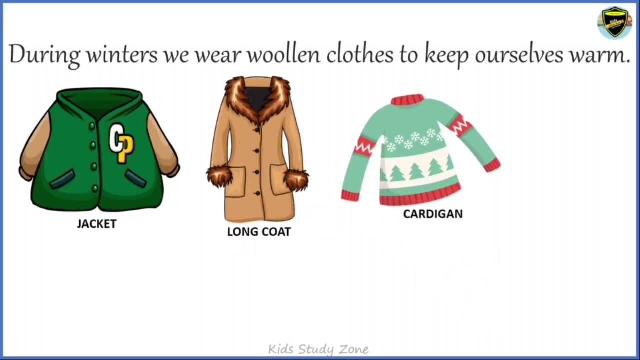 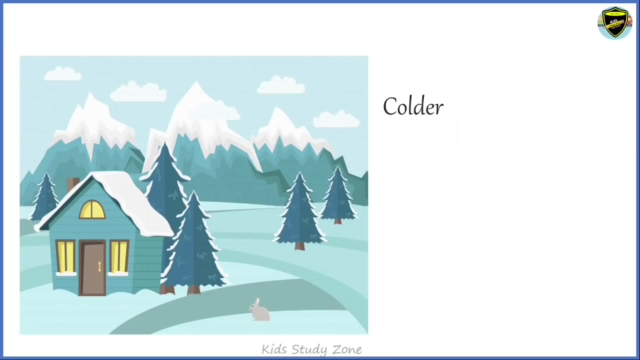 energy to survive adverse weather conditions. During winters, we wear woolen clothes to keep ourselves warm. Let us see some of the winter clothes: Jackfruit Jacket, Long coat, Cardigan, Socks, Mittens, Cap, Muffler. Colder regions have heavy snowfall during winter season. We see lots of snow on ground and trees. 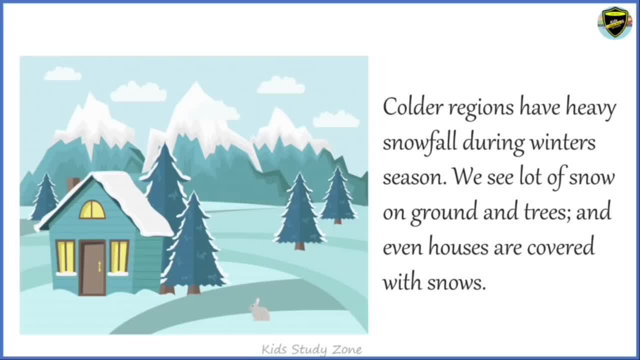 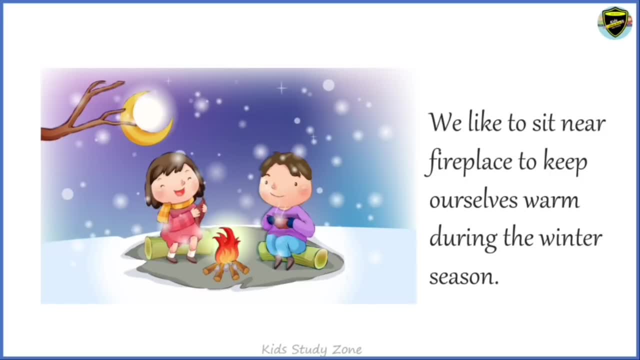 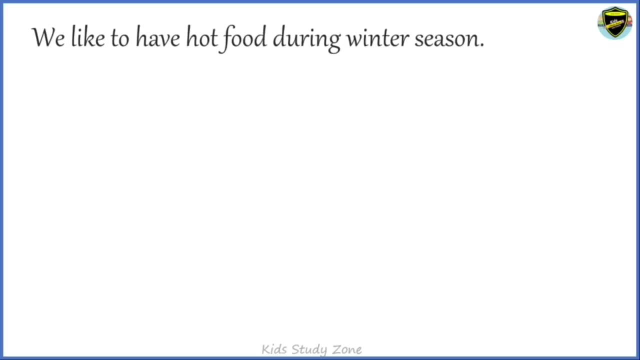 And in winter we see lots of snow on trees. And in winter we see lots of snow on trees And even houses are covered with snows. We like to sit near fireplace to keep ourselves warm during the winter season. We like to have hot food during winter season like coffee, tea and soup. 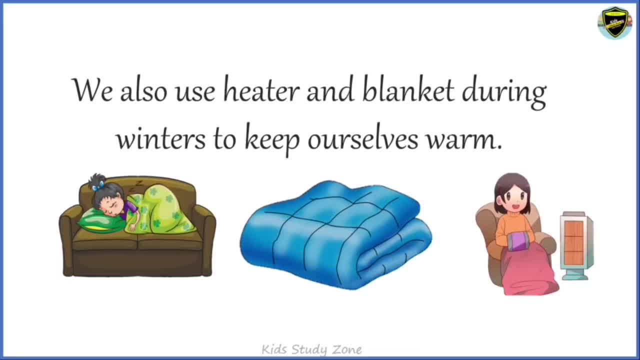 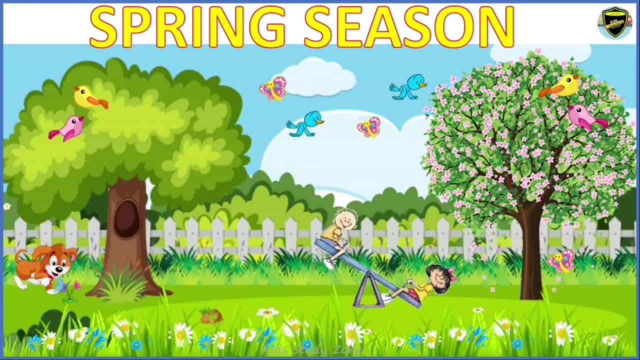 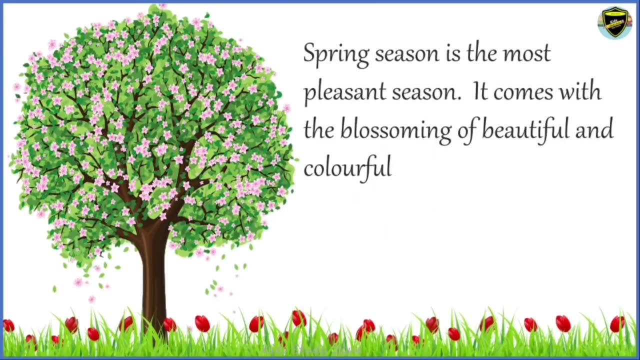 We also use heater and blanket during winter season. But we do not need to wear a blanket during winter. We can keep ourselves warm during winter Spring season. It is the most pleasant season. It comes with the blossoming of beautiful and colorful flowers. 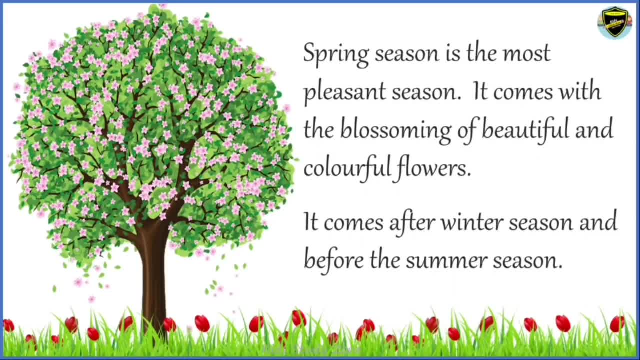 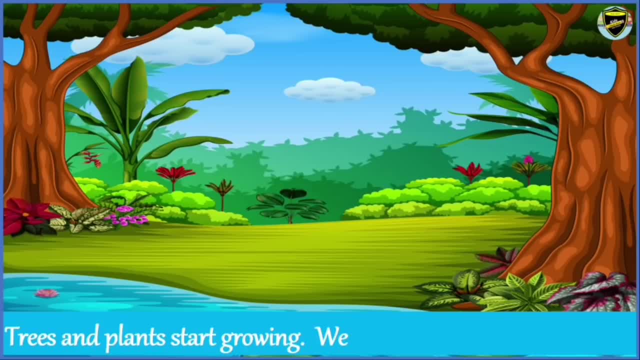 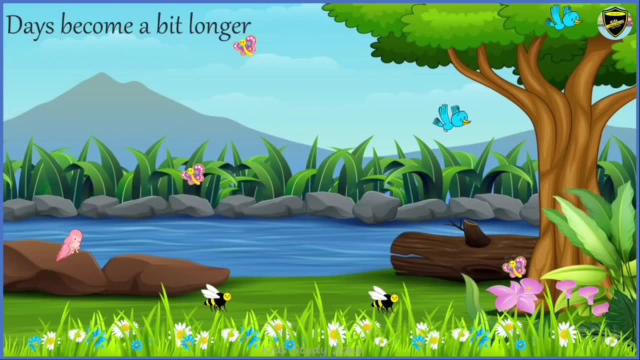 It comes after winter season and before the summer season. After winter season, the trees and plants start growing. We can see greenery everywhere. It is a common scene. We can see greenery everywhere. Days become a bit longer and weather becomes pleasant. 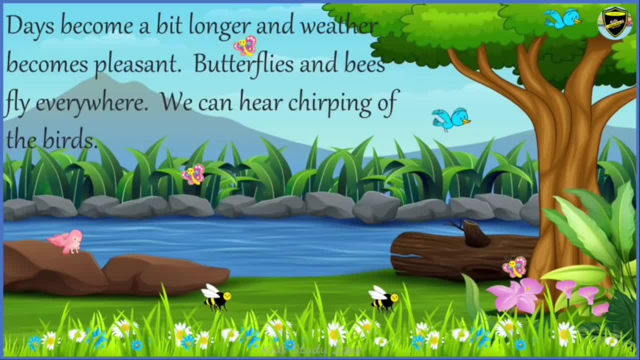 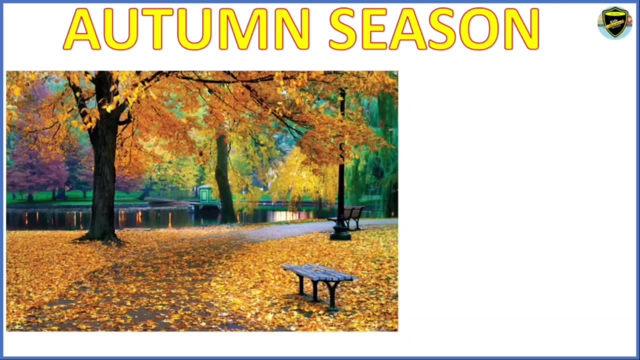 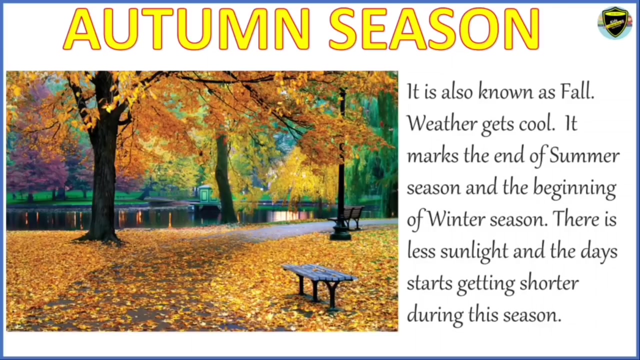 Butterflies and bees fly everywhere. We can hear chirping of the birds. Autumn season- It is also known as fall Weather gets cool. It marks the end of summer season and the beginning of winter season. There is less sunlight and the day starts getting shorter during the season. 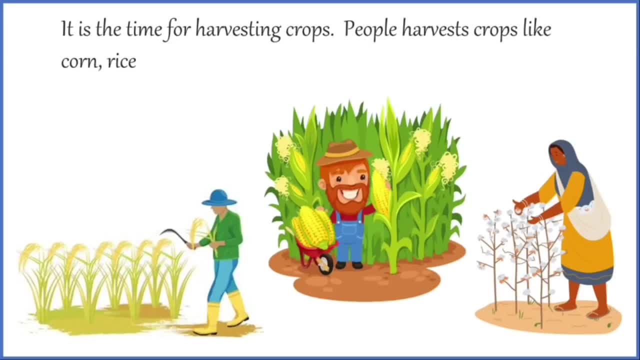 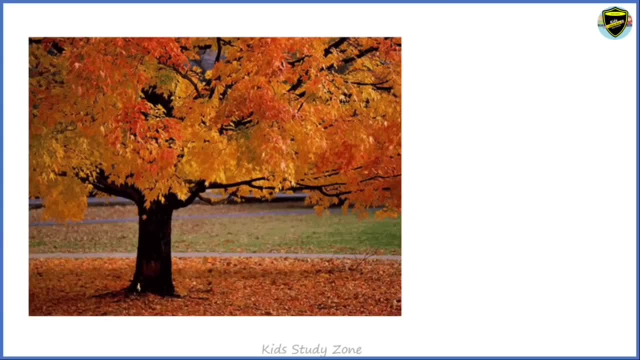 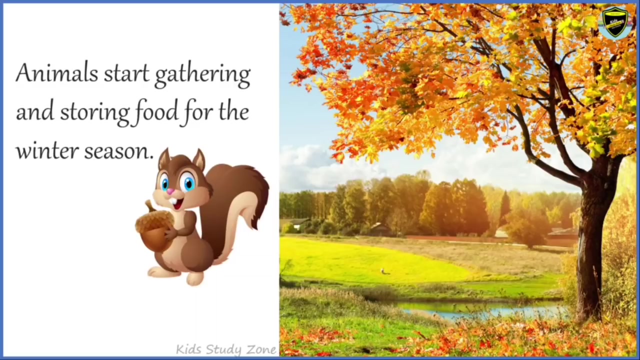 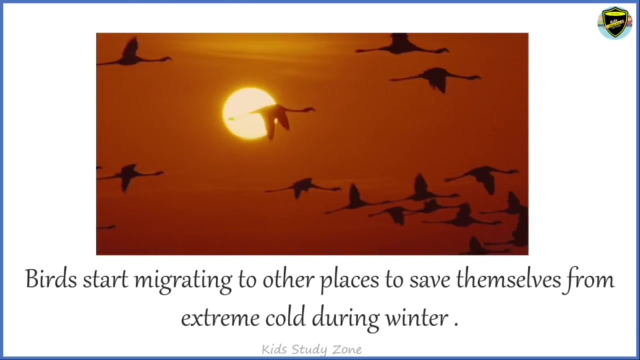 It is the time for harvesting crops. People harvest crops like corn, rice and cotton. Trees start shedding leaves. Most leaves start to change color to red, then yellow and then yellow. Animals start gathering and storing food for the winter season. Birds start migrating to other places to save themselves from extreme cold during winter. 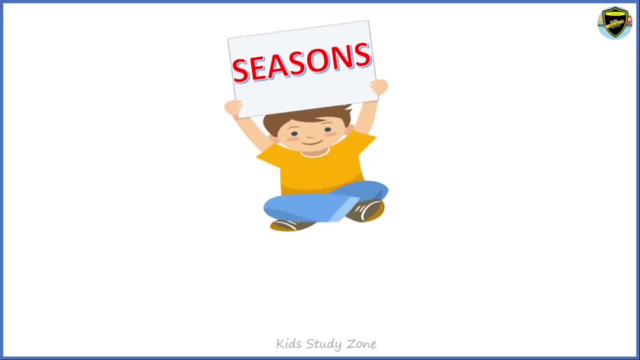 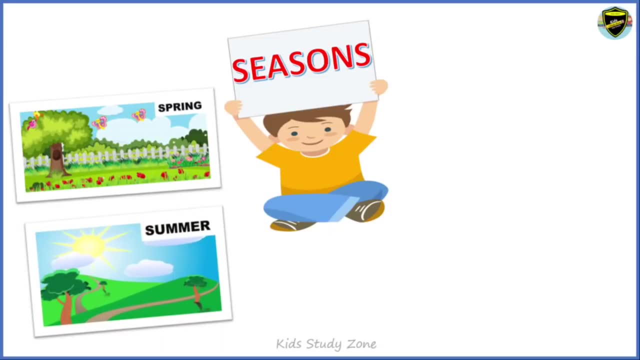 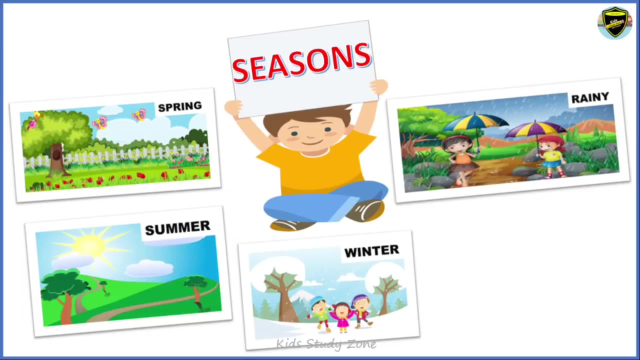 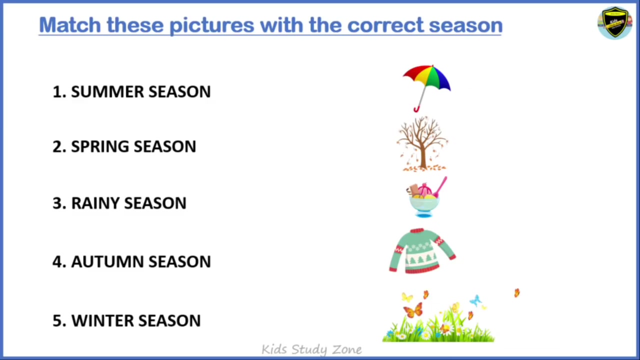 Let us revise the names of all the five seasons once again: Spring, summer, winter, rainy and autumn. Let us do some fun activity to see how much we understood about each season. In this activity you need to match the pictures with the pictures. 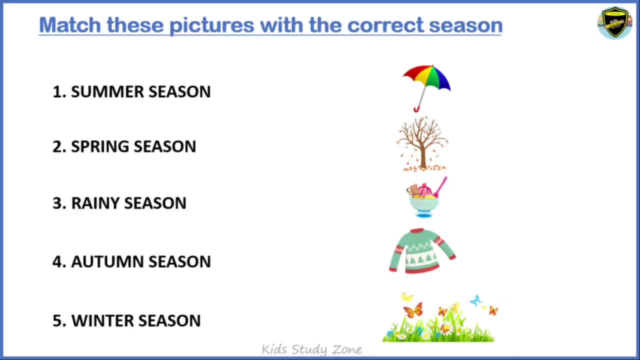 Let us see which is the correct season given to you. On the left hand side you can see the names of various seasons And on the right hand side you can see various pictures and you need to relate them as per the season. Let us see with the first one. 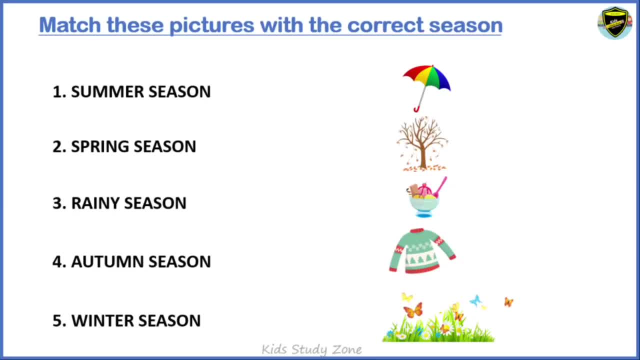 Summer season. Let us see summer season matches with which figure It matches with ice cream, Very good. Next one is spring season. Spring season matches with beautiful flowers, butterflies. Next one is rainy season. In rainy season, we see people with umbrellas. 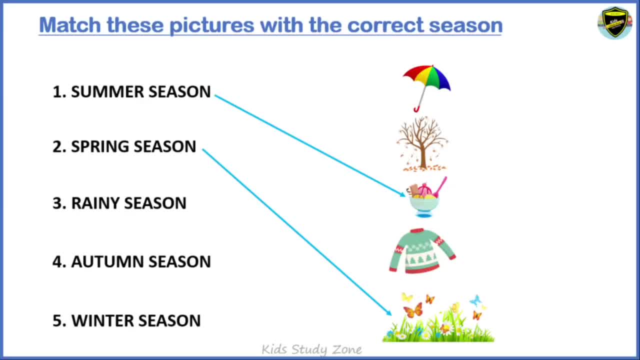 Very good. Next one is winter season: People with umbrellas- Very good. Next one is winter season: People with umbrellas. People with umbrellas. During the winter season, we see leaves falling. Another one is autumn season. During autumn season, we see leaves falling. 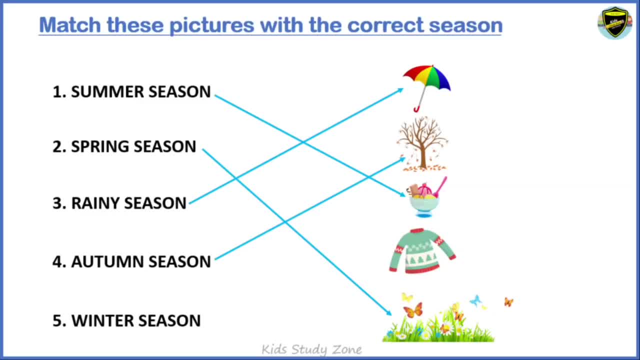 That's right. Then winter season: During winter season, we use cardigans. Excellent, children. Now let's do some more activity. Now, let's do some more activity. In this, you need to take the correct option. Question number one is: 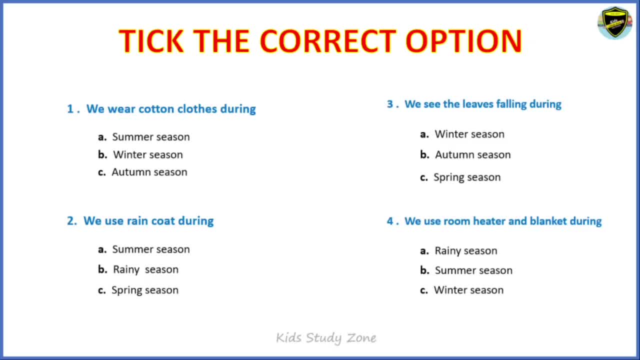 Question number one is: We wear cotton clothes during. options are summer, winter and autumn. The correct answer is summer season. Next one: we use raincoat during summer season, rainy season or spring season. The correct answer is rainy season. 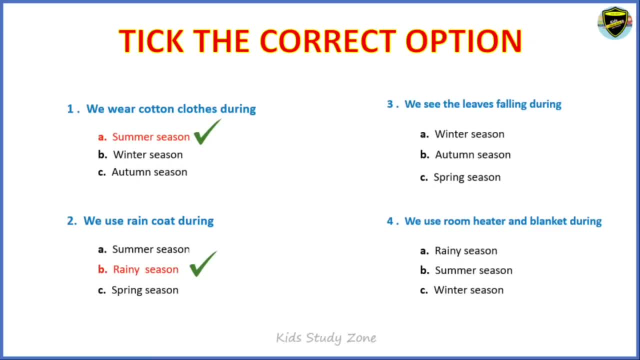 Very good. Third question is: we see leaves falling during. options are winter season, autumn season or spring season, And the correct answer is autumn season. Fourth one is: we use room temperature, Room heater and blanket during options are rainy season, summer season and winter season. 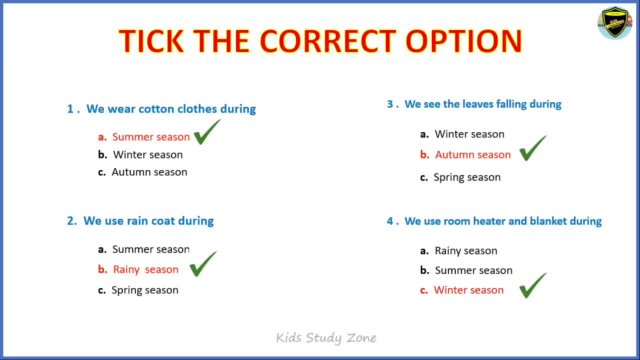 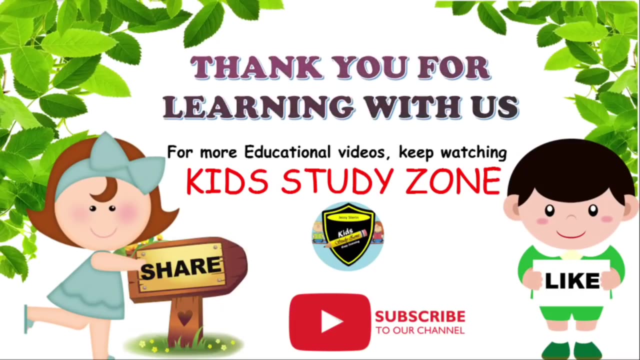